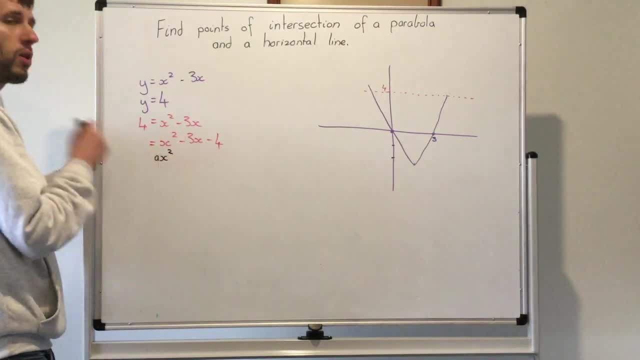 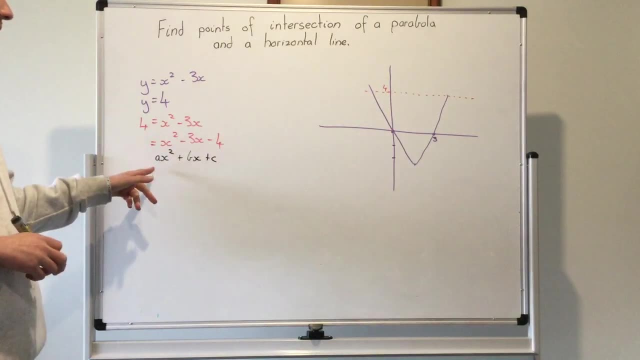 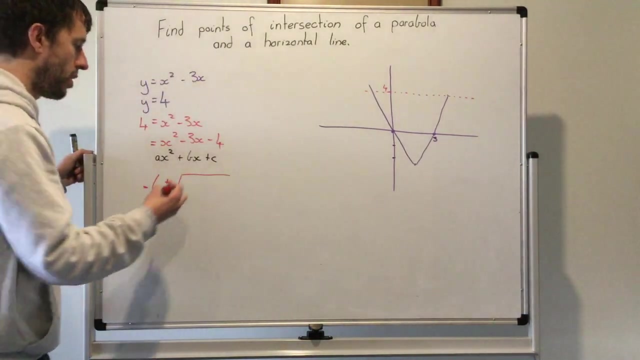 So just remember: our equation is ax squared plus bx plus c, And that just means a is equal to 1,, b is equal to negative 3, and c is equal to negative 4.. Our quadratic equation is negative: b plus or minus the square root of b squared minus 4ac divided by 2a. 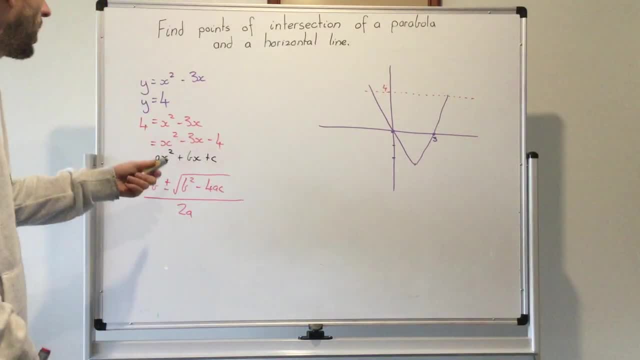 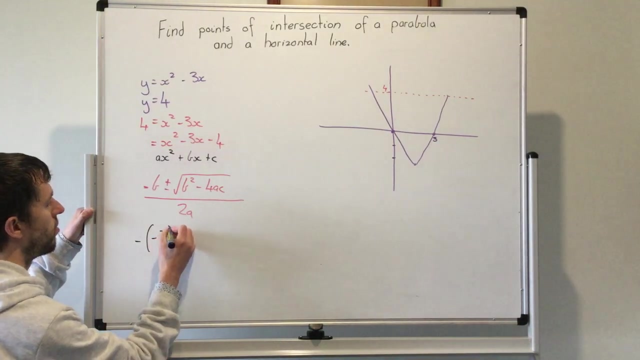 If you don't know where that equation comes from, please go back and look at the quadratic equation proof. So all I need to do now is I'm going to substitute my values in, So negative at my, b is negative 3 plus or minus, and that's just because we've got a square root. 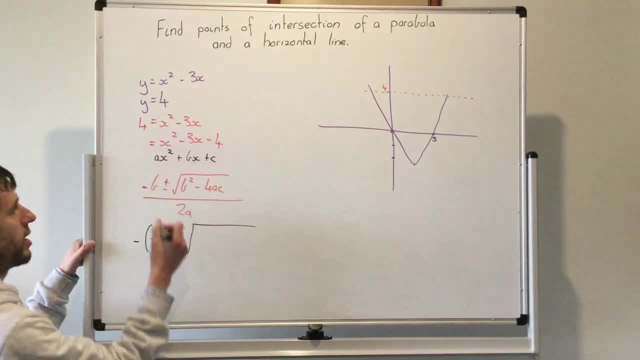 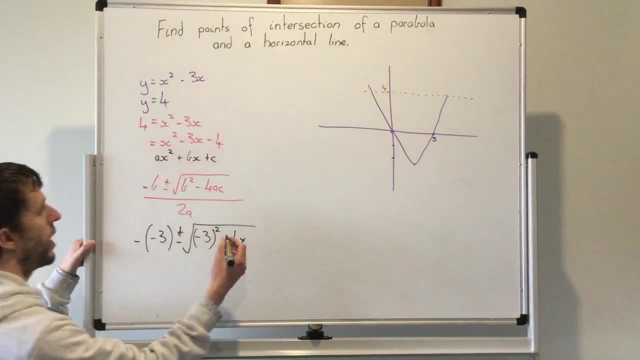 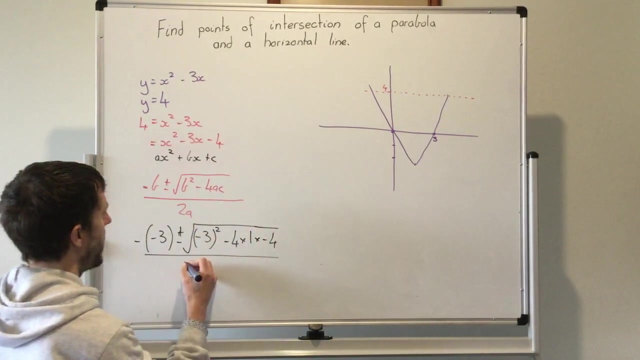 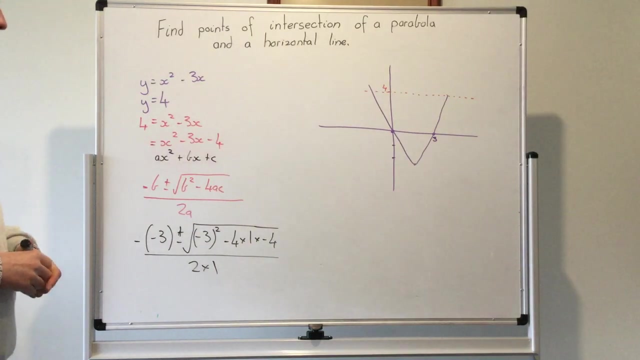 b squared b, negative 3, negative 3 squared minus 4 times a is 1 times c, which is negative Negative 4 divided by 2 times a, Again a is just 1.. So we can simplify our equation. 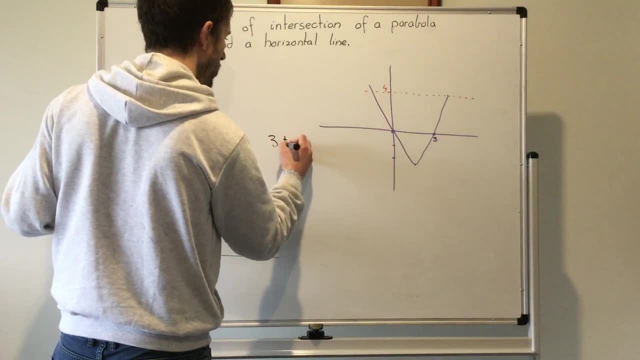 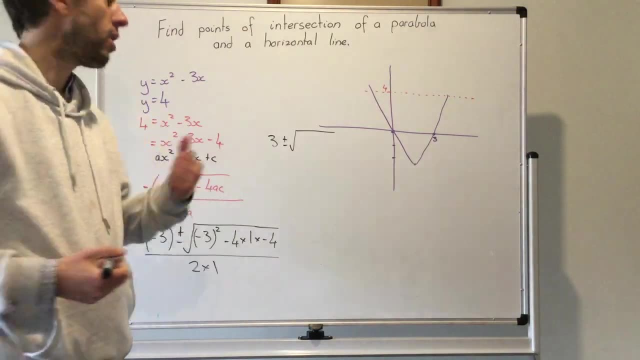 Negative and negative equals a positive, So I've got 3 plus or minus negative 3 squared Well, negative and negative equals a positive. 3 times 3 is 9.. And I've got minus. 4 times 1 is just minus 4.. 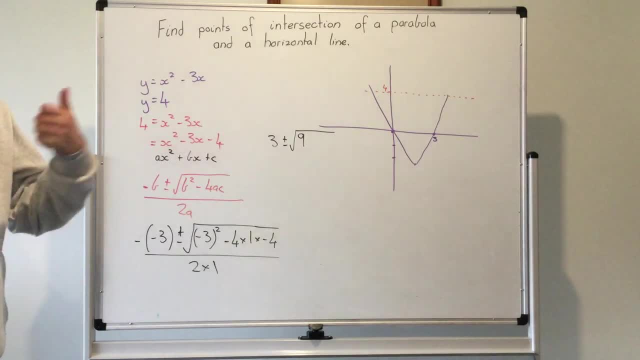 Minus 4 times another minus 4 is a positive, and 4 times 4 is 16.. So it becomes plus 16.. Divide it by 2 times 1.. Well, 2 times 1 is just 2.. 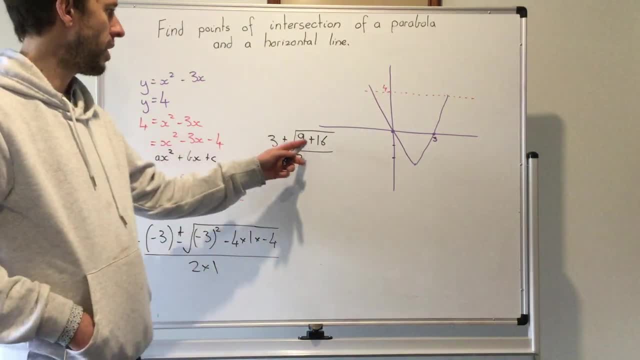 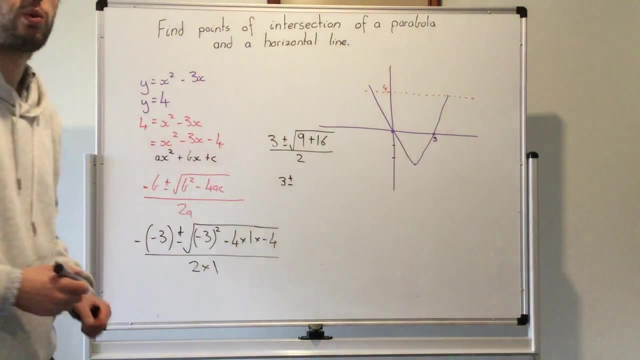 So we've simplified it. I'll go one step further: 9 plus 16, that's 25.. If I've got the square root of 25, that just means 2 numbers that times together that equals 25 will be 5.. 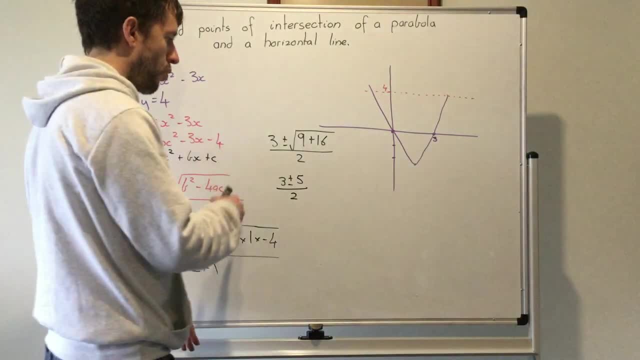 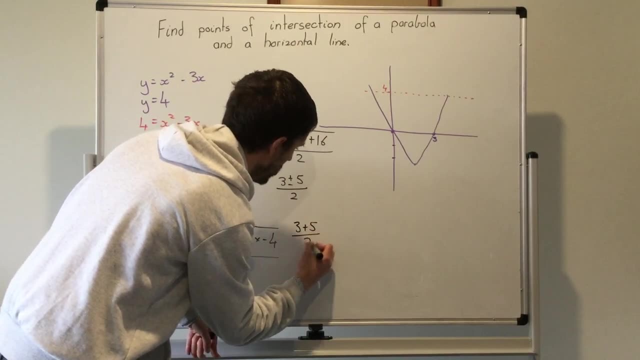 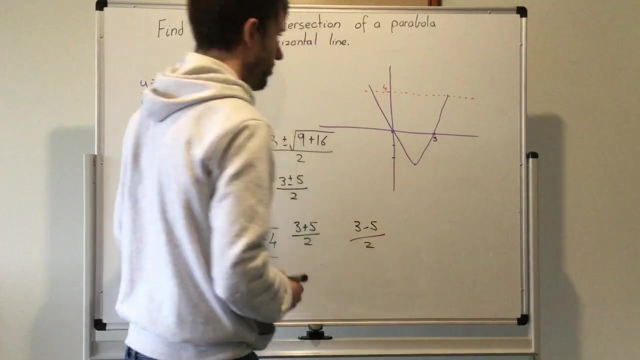 So that gives me 2 x values. One will be 3 plus 5, equals 3 plus 5 divided by 2. And the other one will be 3 minus 5 divided by 2.. So let's have a look. 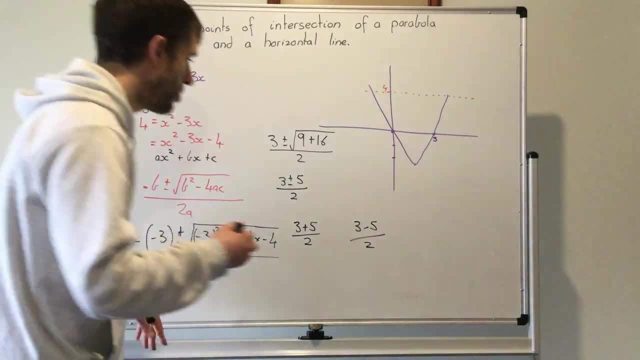 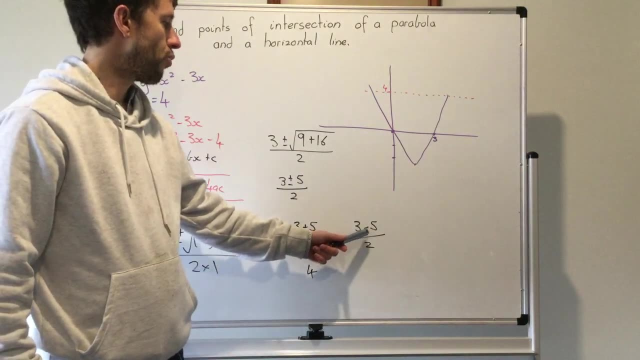 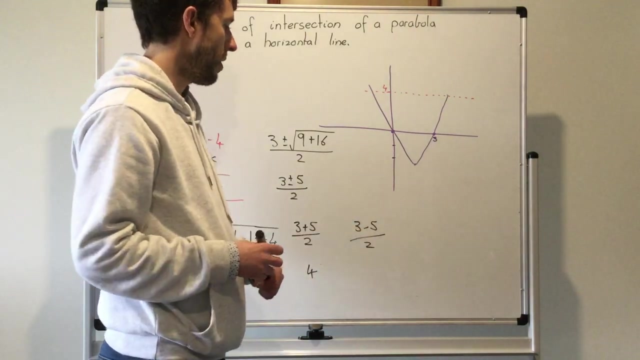 3 plus 5.. 5 is 8.. 8 divided by 2 is 4.. And we've also got 3 minus 5.. 3 minus 5 is negative 2.. Negative 2 divided by 2 is negative 1.. 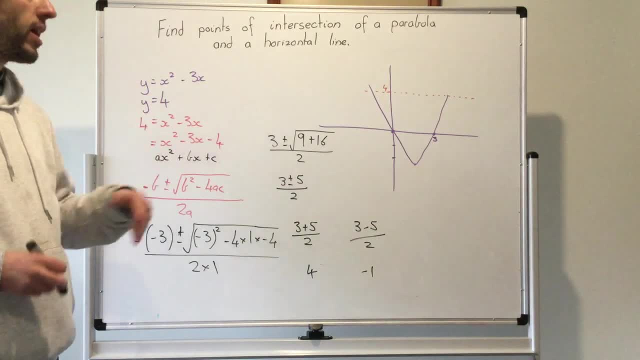 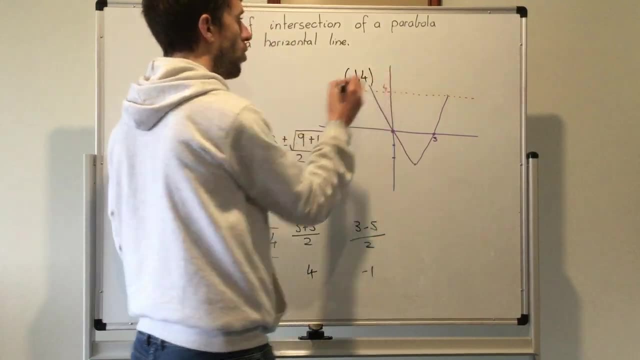 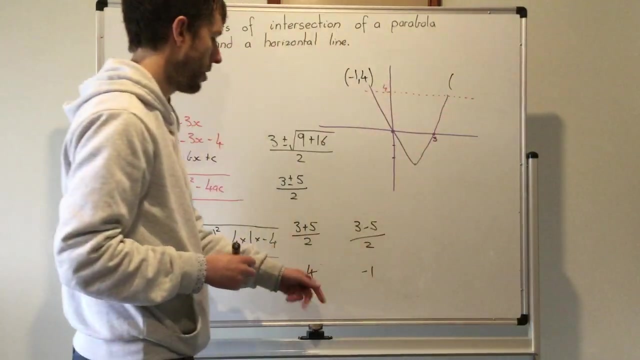 So from every 25 points for when they cross, I know that when x is negative 1, then y is 4, is one point. And the second point that I have is when x is 4, and y is 4, it's going to cross. 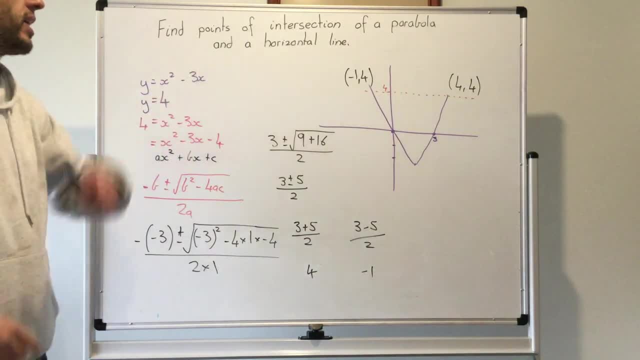 If you need any action, help with finding points of when a line intersects a parabola, feel free to get back to me and I'll make a video just for you. Oxygen. Whenever we hear the word oxygen, what is the first thing that comes to your mind? Trees, right, But did you know that the oceans produce more than 50% of the oxygen on our planet? All thanks to a little organism known as plankton. All ocean ecosystems contain marine plankton. 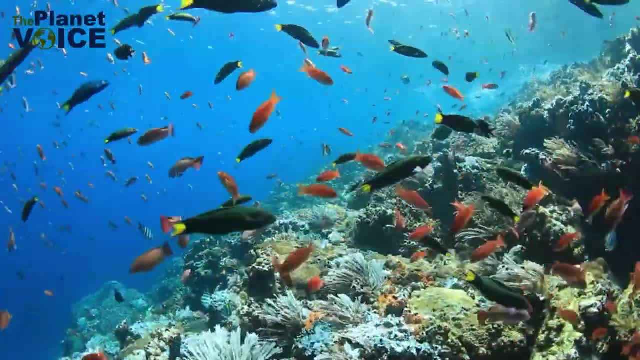 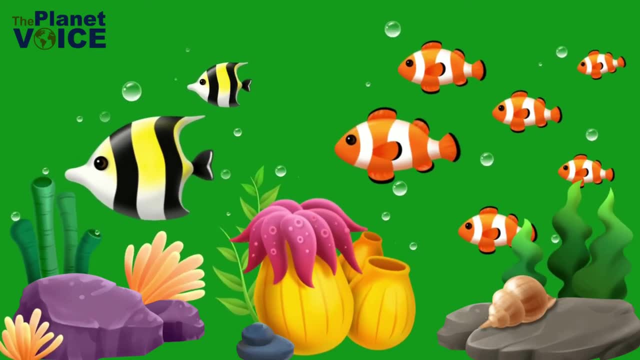 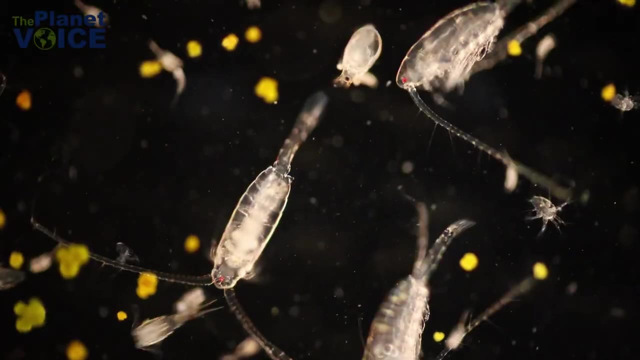 which is essential to preserving the harmony and health of the ocean and its intricate food webs. The oxygen, nutrients and biomass they produce also support terrestrial life, from the food we consume to the air we breathe: Phytoplankton, which are plants, and zooplankton. 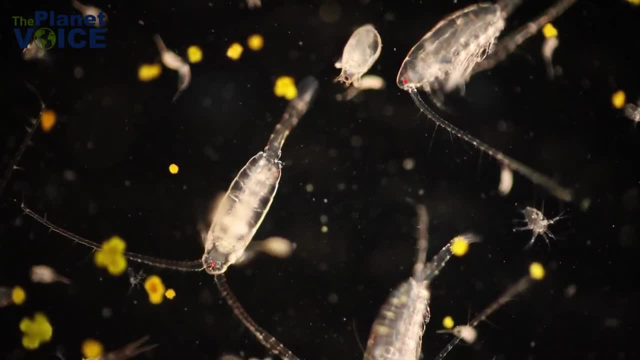 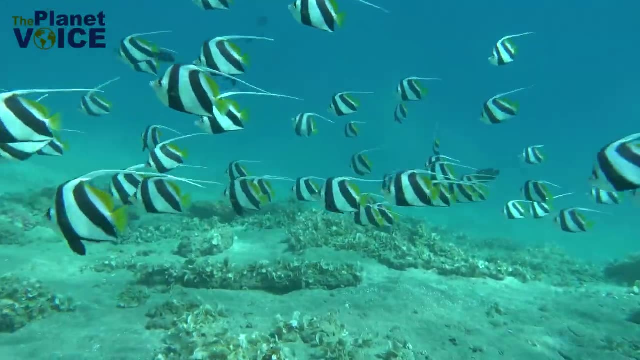 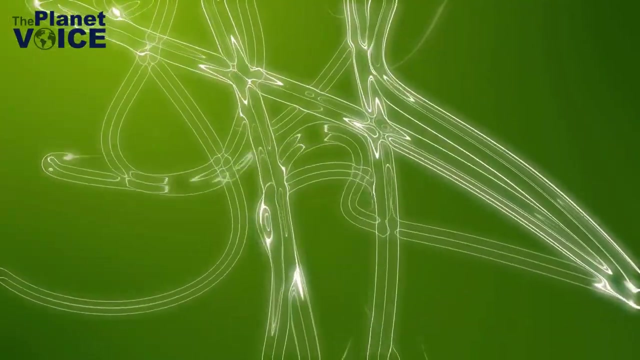 which are animals, are the two main categories of plankton. Zooplankton and other tiny marine organisms consume phytoplankton, which is then used as food by larger species like fish and crustaceans. Photosynthesis- Photosynthesis is the process through which phytoplankton grows. 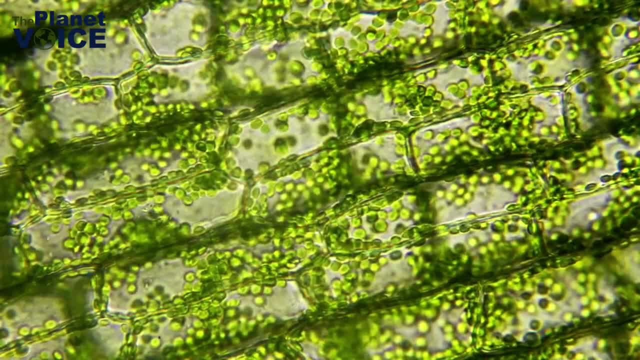 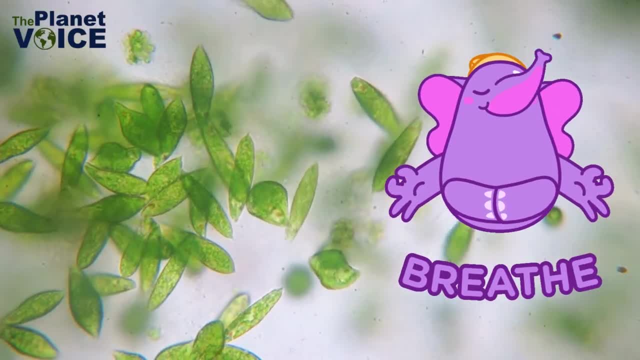 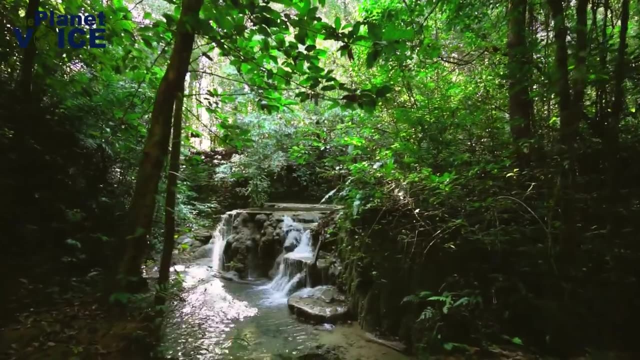 Oxygen is released into the water by phytoplankton during the process of photosynthesis. Since the oceans cover 71% of the planet, phytoplankton are in charge of producing up to 50% of the oxygen that humans breathe. Trees, bushes, grasses and other plants that grow on land use photosynthesis to produce the